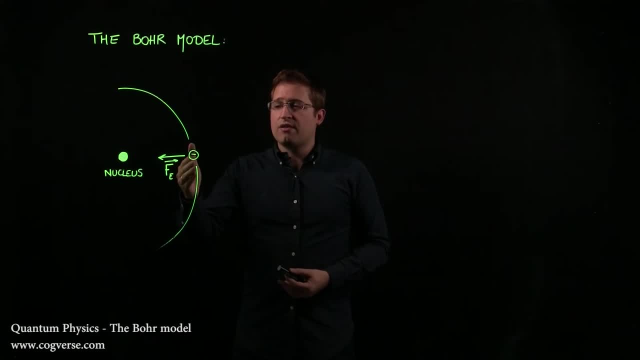 with a frequency equal to the frequency of revolution, And if it emits a wave, it loses energy. If it loses energy, the orbit gets smaller and your frequency decreases continuously, And therefore you have a wave with a continuously decrease in frequency. 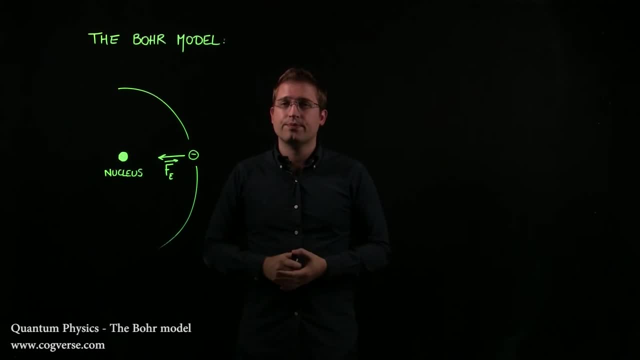 and you get a continuous spectrum, not a line spectrum. So that didn't really work. But Bohr came around and said: well, hold on, I like the idea of an electron orbiting the nucleus. Let's say, maybe, that there are different orbits. 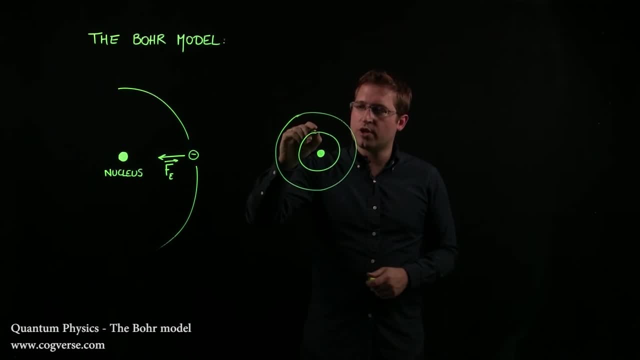 There are stable orbits that are allowed, Stable orbits on which the electron is allowed to stay without radiating anything, And the only time it would radiate is when it goes from one stable orbit to another, And that happens when it absorbs a photon or it emits a photon. 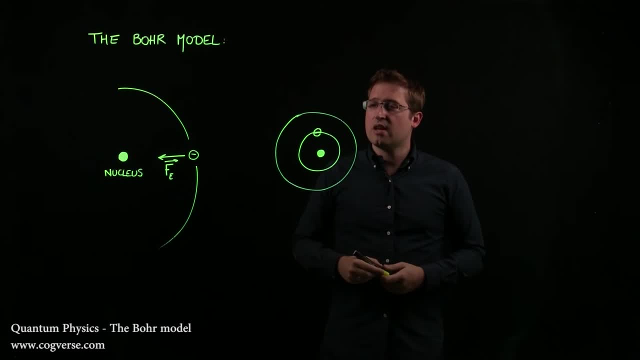 It's spontaneous absorption or spontaneous emission, And therefore, if a photon came around with exactly the energy equal to the difference in energy between these two orbits, then the electron could jump onto this stable orbit, And once it gets there it doesn't radiate, And that would work. Now, that's a very bold idea. 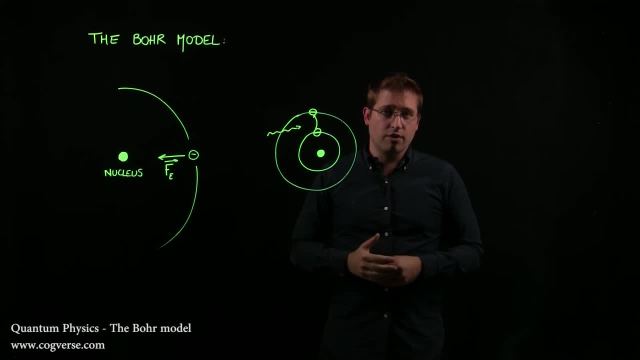 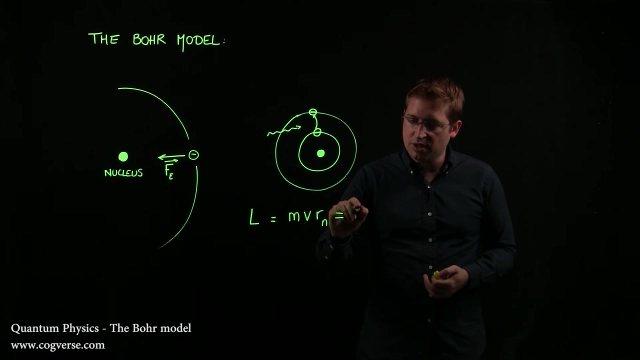 And in order to give a formula for the radii, Bohr suggested that the angular momentum of the electron had to be quantized. The angular momentum is mv r sub n, And he suggested that it had to be equal to n times h bar, which is n times h, Planck's constant. 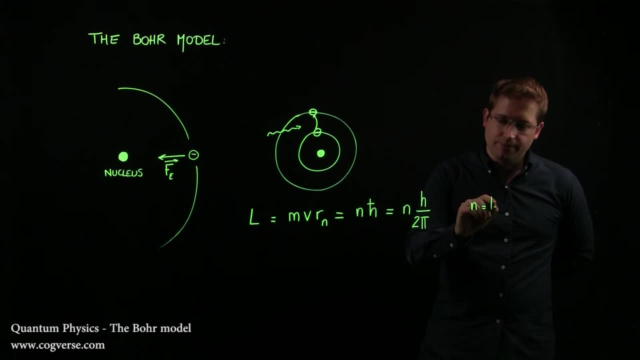 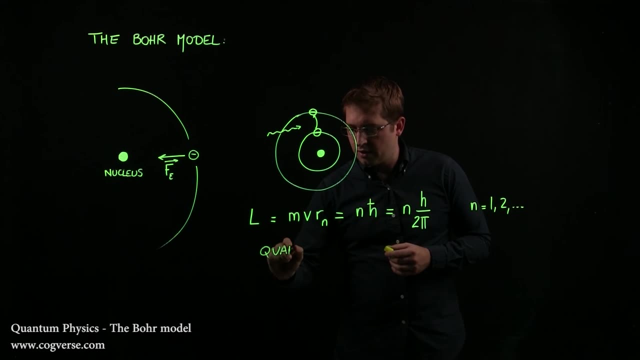 divided by 2 pi. Of course, this for n equal 1,, 2, et cetera, And this is called the quantization condition. quantization condition, And along with the model of the electron orbiting the nucleus, with the electrical force pulling it. 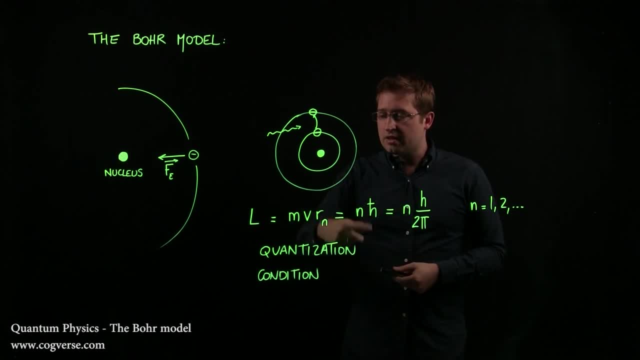 inward so that it has a circular orbit. This gives you the expression of the different radii for the stable orbits And, as it happens, the energy levels that are derived from that give you wavelengths that exactly match what you have in your hologram. And because we're using the natural